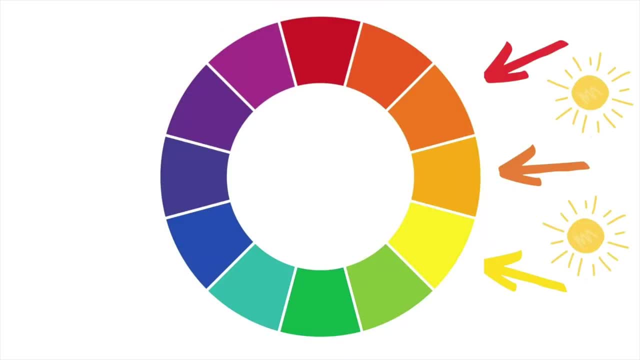 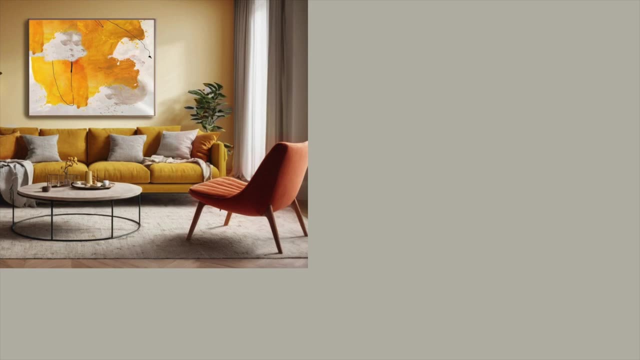 virtually make every single color in the world. Warm colors include reds, oranges and yellows, as well as earth tones such as browns and tans. And warm colors tend to be a little bit more vibrant and energizing, which are great for living rooms or any space really where you want to make. 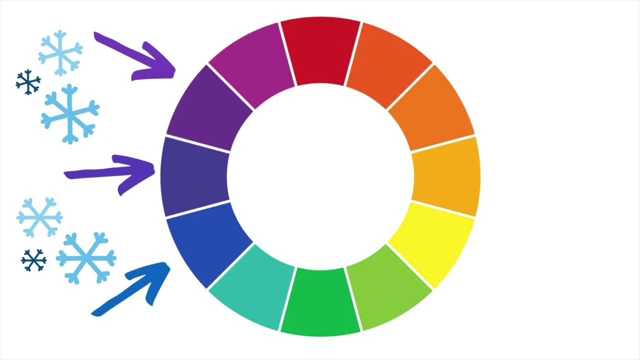 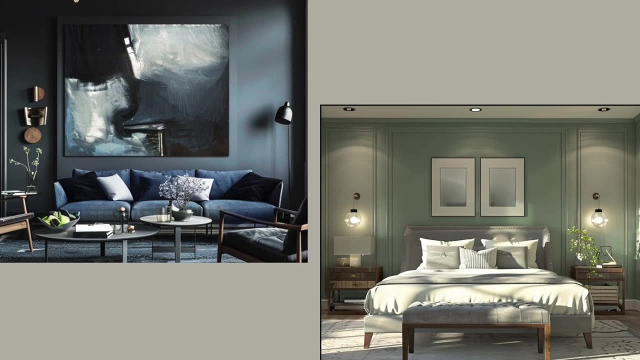 something more welcoming and exciting. Okay, now your cool colors, which are your blues, your greens and your purples, and they can give you more of a soothing and calming effect, Like if you use a blue or soft green. these are ideal for bedrooms or really anywhere where you want more of a 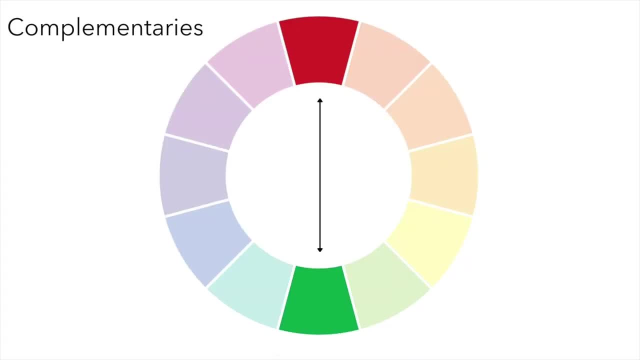 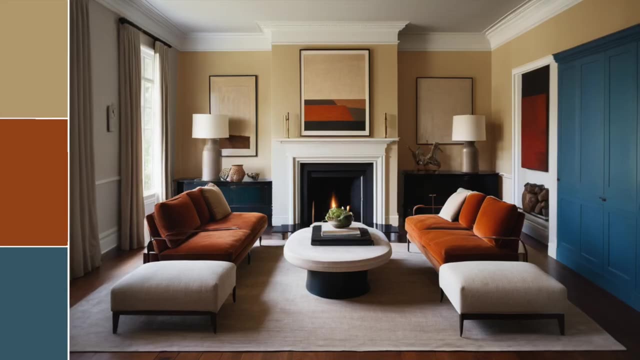 soothing and calming effect. Then you have your complementary colors, which are colors that are opposite each other in the color wheel And because they're opposite each other, they have very, very high contrast. So if you want a color to really pop or you want to increase its vibrancy and its, 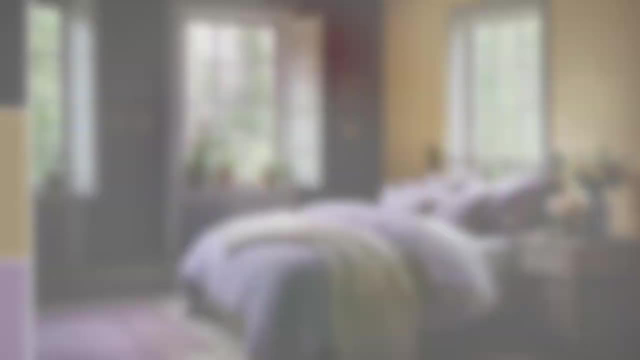 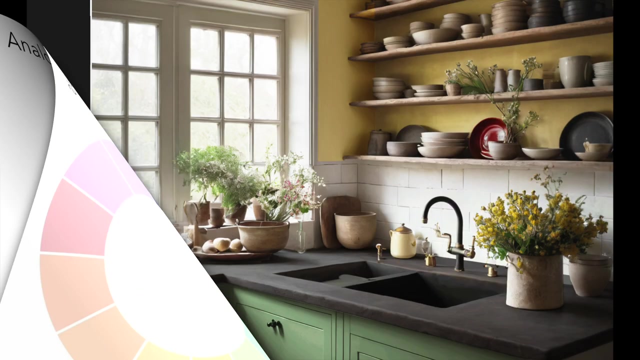 intensity, then place it against its complementary colors. Analogous colors are groups of three colors that are next to each other in the color wheel And because these colors are basically neighbors, they share a base color in their mix, which ensures that the scheme is visually pleasing and. 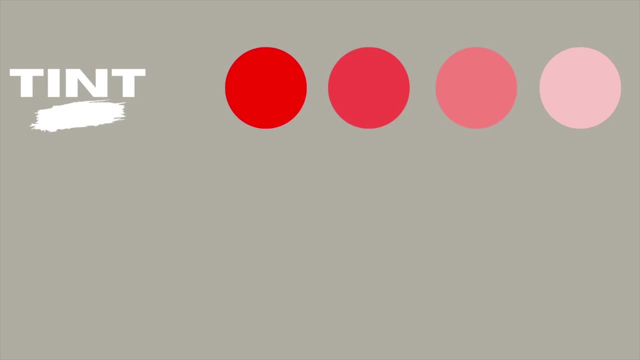 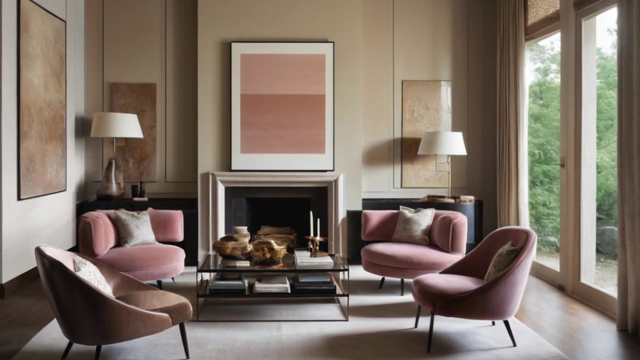 harmonious Tint is the variation of a color by adding white. The higher the tint, the more white you're adding to a color and therefore it becomes brighter. This gives you more of a delicate and softer appearance. Tone refers to a color that has been softened or toned down by adding gray. 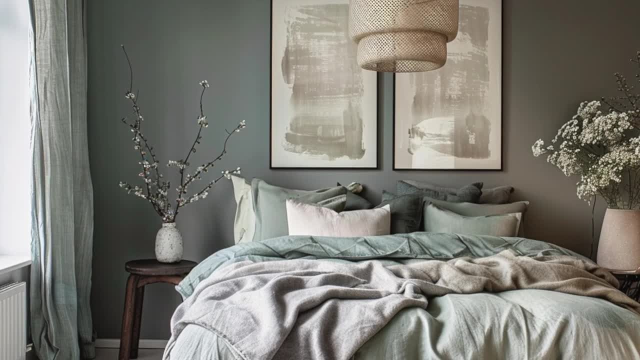 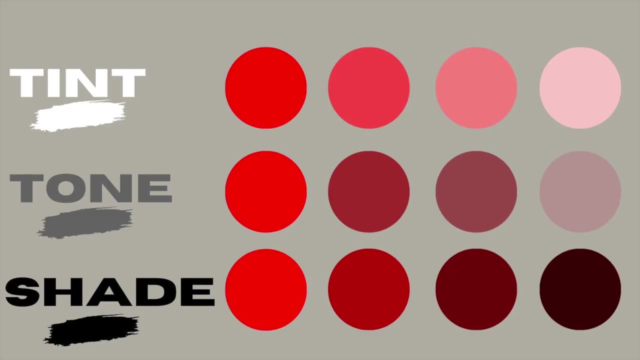 making it less intense and more muted than its original. color Tones are excellent for creating contrast, but also fantastic choices for background colors. And then shade is the variation of a color by adding black. The higher the shade, the more black it has, And this is where chroma comes in. 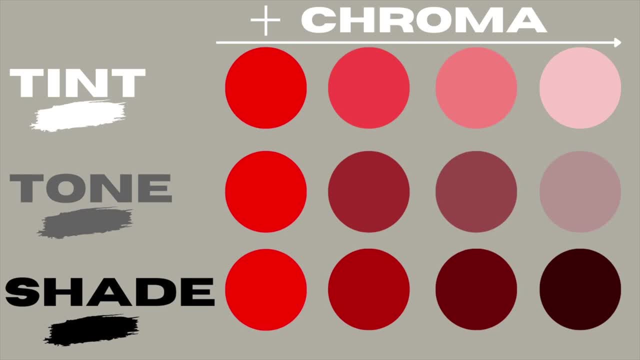 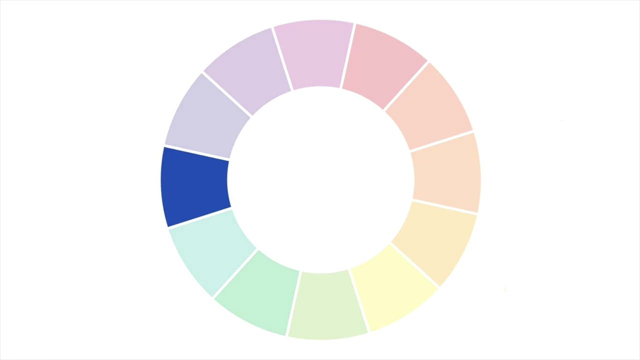 The higher the chroma, the more pure and vivid a color is, And then the lower the chroma, the more dull or muted the color will be. Adding, white, gray or black will lower the chroma of a color- Think of slate, grays, neutrals and pastels. Then from chroma you get monochromatic color palettes. 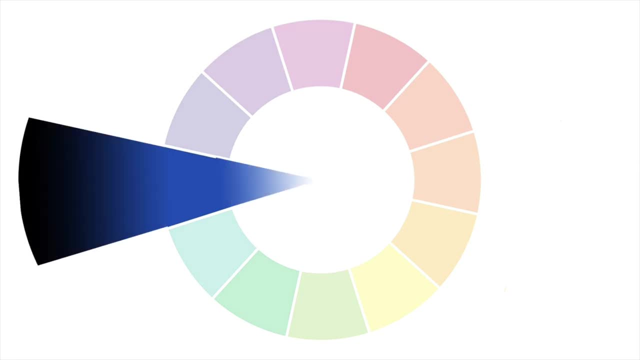 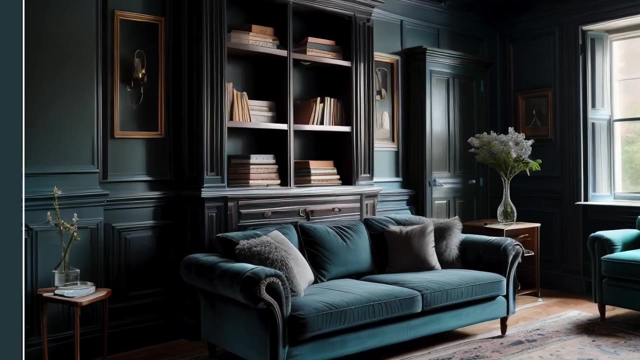 which involves selecting a single base color and then adding more chroma to the color- And this is color- and using its variations of shades, tints and tones, You're basically layering colors in different intensities and saturations to add richness to the space. They can create a very 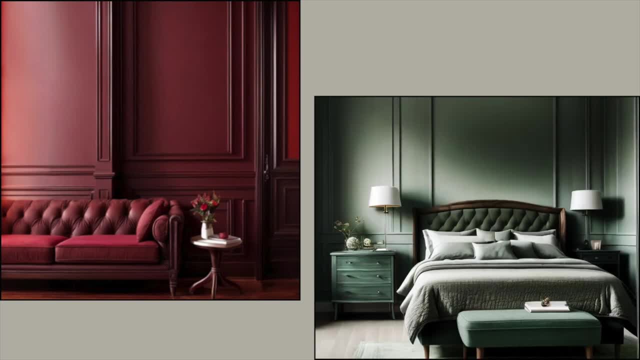 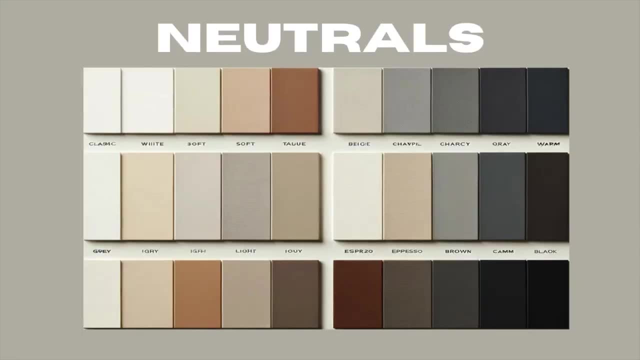 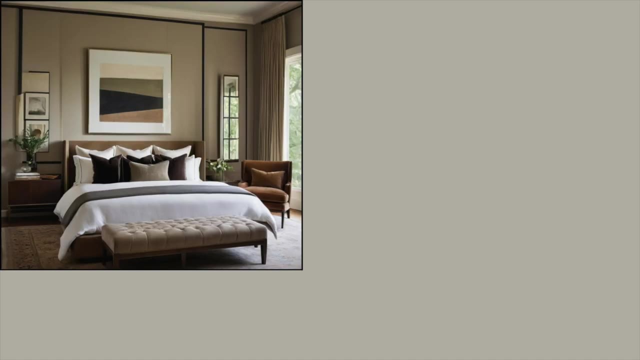 cohesive and unified look which can be soothing but also very striking and elegant at the same time. Neutrals include white, black and grays, also beiges or any color really with low saturation or low chroma. They are essentials as they can act as calming backgrounds to any room. They can also 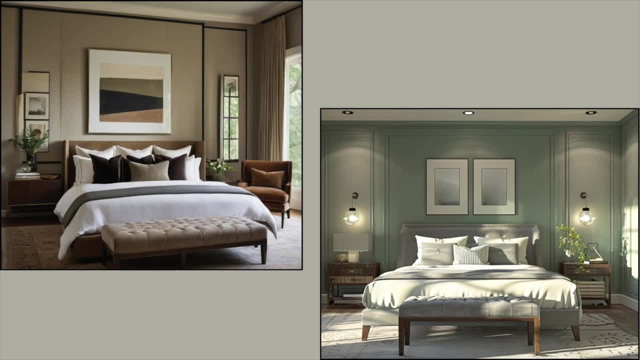 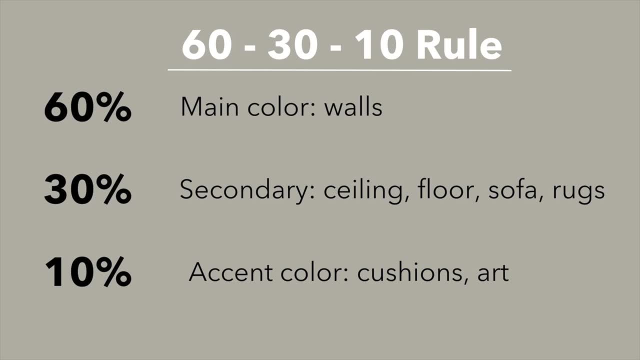 act as bridges or connectors between other more vibrant colors, giving you more breathing space to play around. The 60-30-10 rule is when you use 60% of a dominant color and then 30% of a secondary color and then 10% of an accent color. It's a classic principle which creates hierarchy. 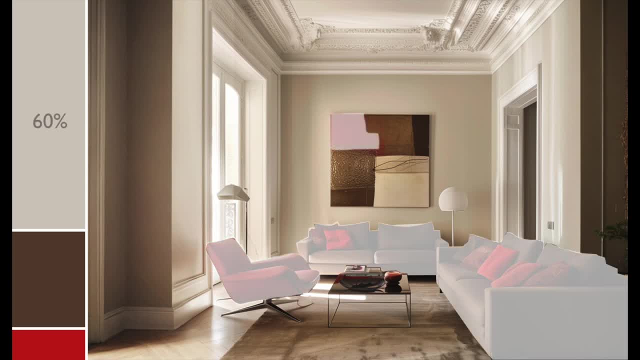 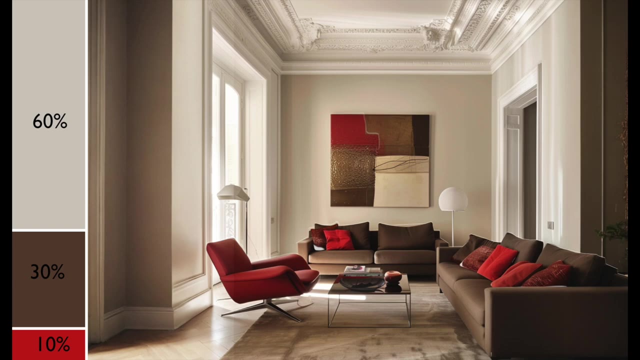 that gives you more of a balanced and visually appealing interior. For example, use 60% of a neutral color for walls or ceilings, 30% of a base color for sofas, curtains and rugs, and then 10% for an accent color in pillows, vases, art or any small moment that can give you a pop of color. 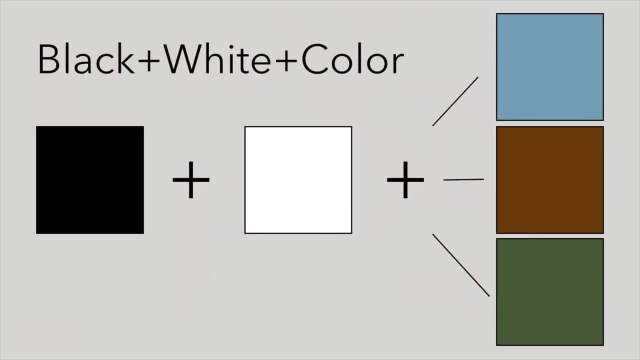 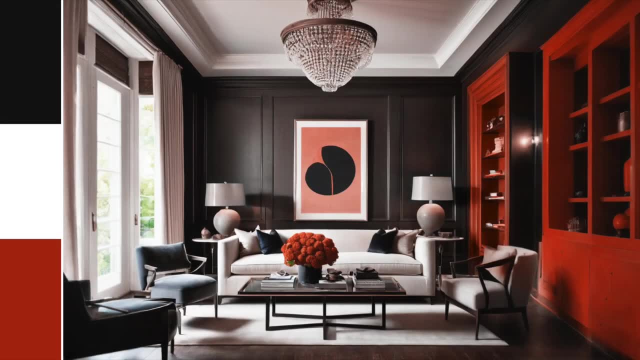 Okay, now let's get into the fun stuff by looking at some beautiful images of different color palettes that you can actually use in your home. The combination of black, white and a distinct color is a classic and powerful strategy that creates visually striking spaces. 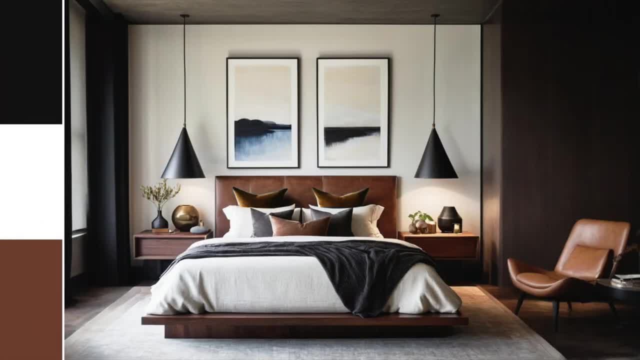 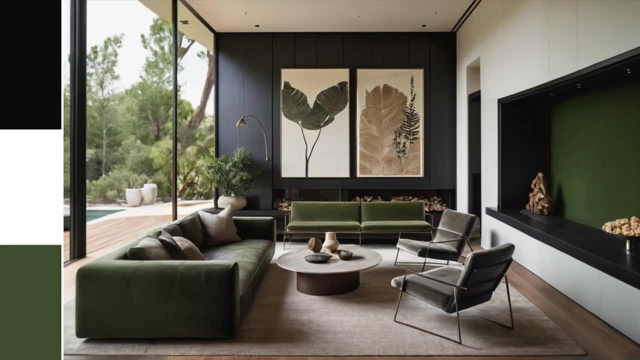 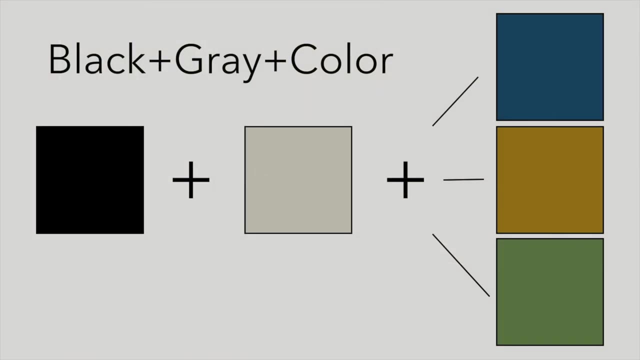 The high contrast between the black and the white creates a dynamic and visually compelling foundation that can make any space feel more modern and elegant, And introducing a specific color adds depth, interest and personality. Combining black gray and a color provides a neutral backdrop that is both elegant and 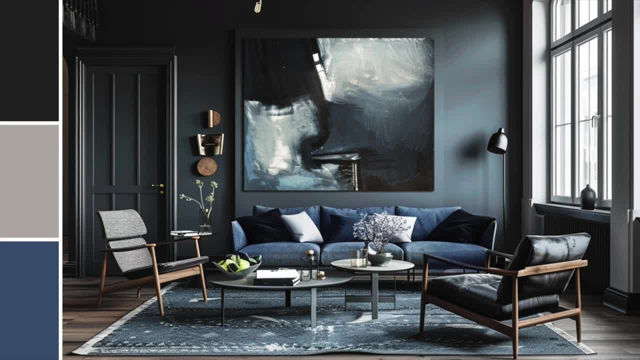 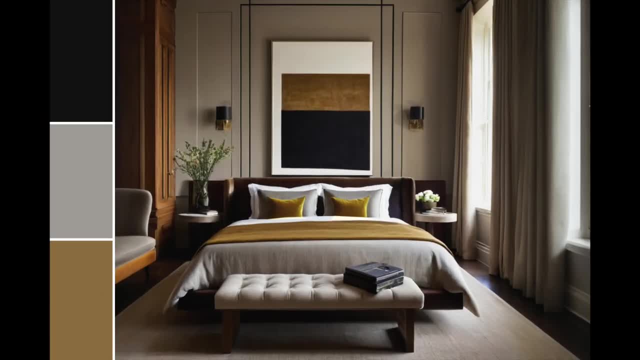 understated. Black adds depth and definition, while gray serves, as you know, more of a softening intermediary, bridging the stark contrast between the black and whatever accent color you choose to add. This creates a harmonious and balanced look that is easier on the eye than a sharper contrast. 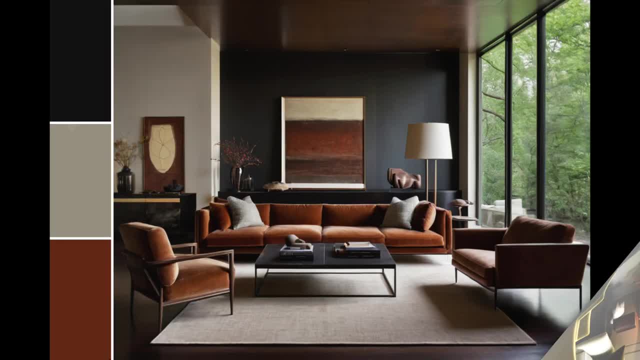 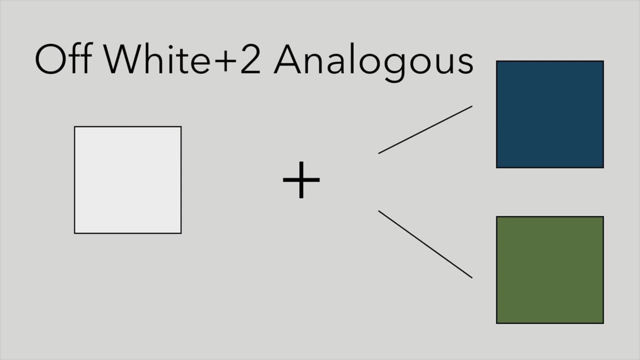 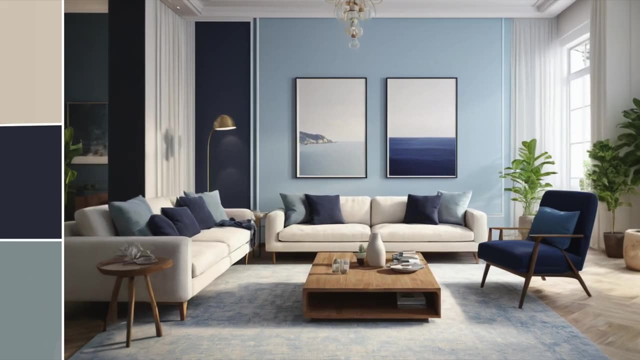 of black and white, SUPP tempted. The combination of off-white and two analogous colors creates a more harmonious and soothing palette that can bring warmth and subtlety to any space. This approach leads towards a more natural and cohesive and dewier look by using colors that sit next to each other in the color wheel. 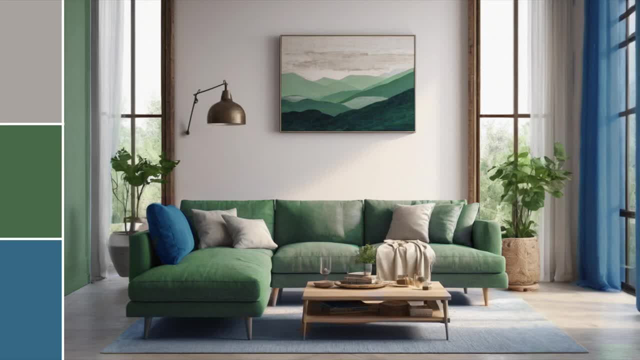 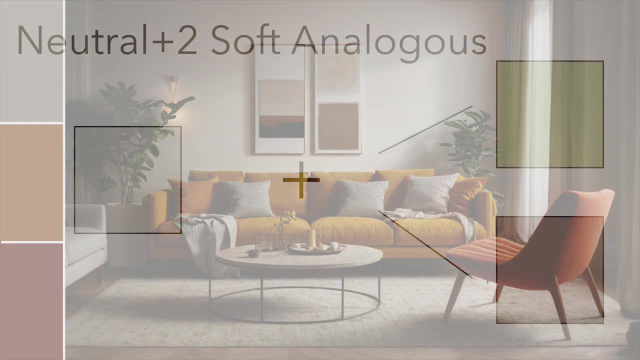 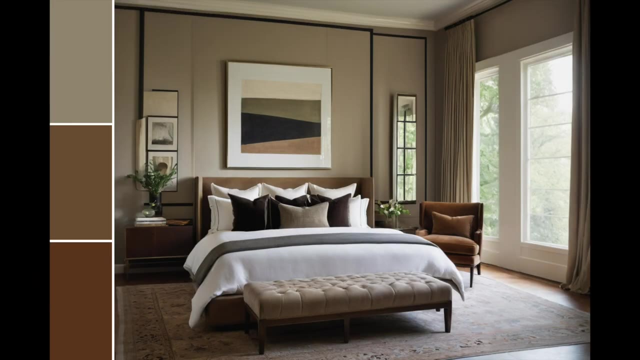 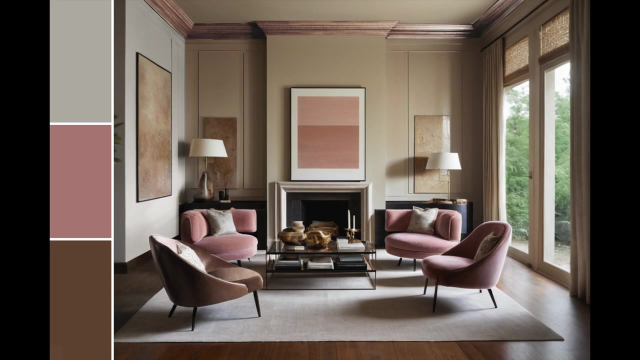 Vital Radical PhD. Always Be strangers. Combining a neutral base with two soft analogous colors creates a tranquil and cohesive environment that's both inviting and visually appealing. This approach enhances the calming qualities of analogous colors while also grounding the scheme with a versatile neutral. This color scheme is great for you know, bedrooms or wherever you want a softer and 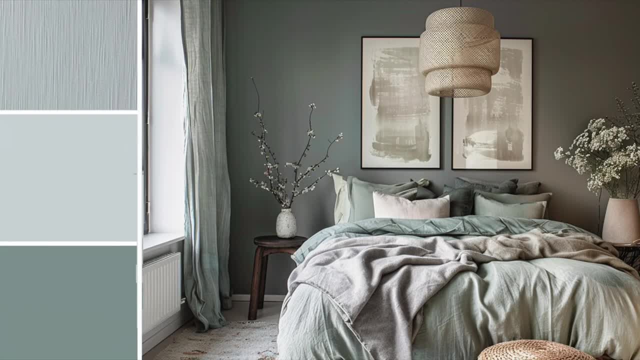 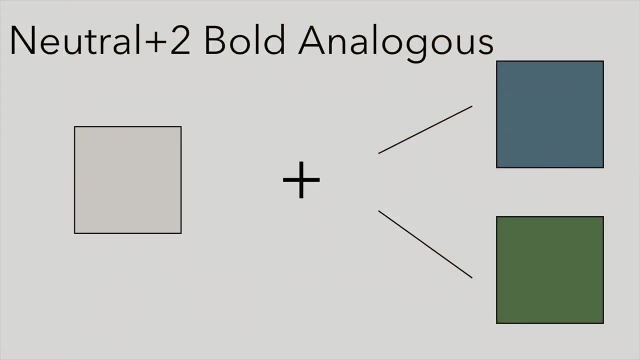 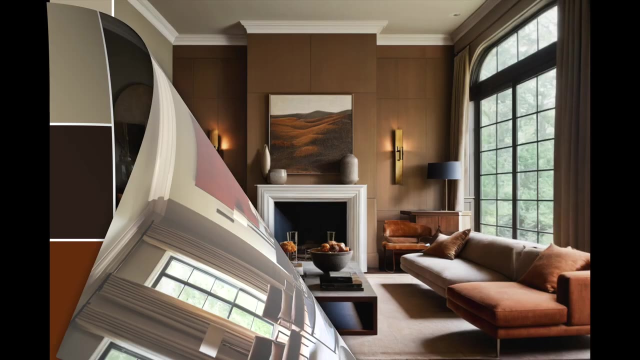 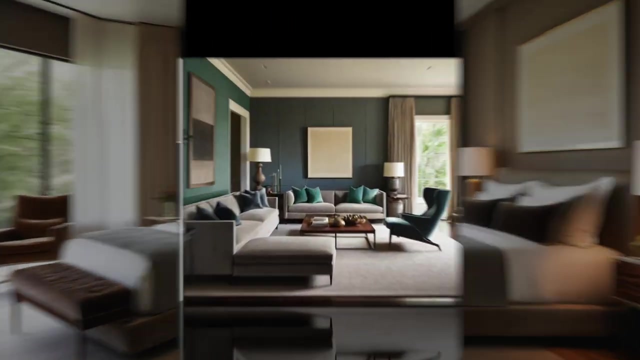 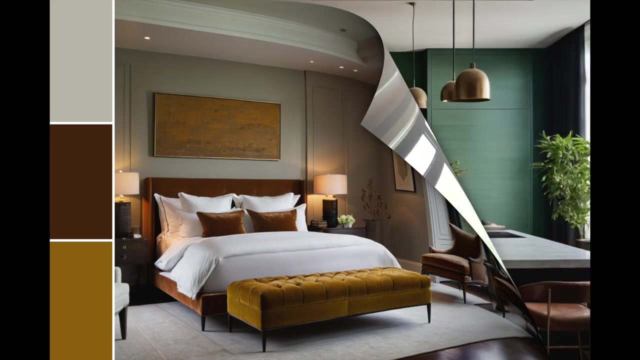 more airier look. Incorporating a neutral base with two bold analogous colors can create a dynamic but balanced aesthetic that combines the grounding effect of the neutrals on the one hand, with the vibrancy and the energy of bold colors on the other side. This approach allows for a playful yet sophisticated space that can adapt to many styles and preferences. 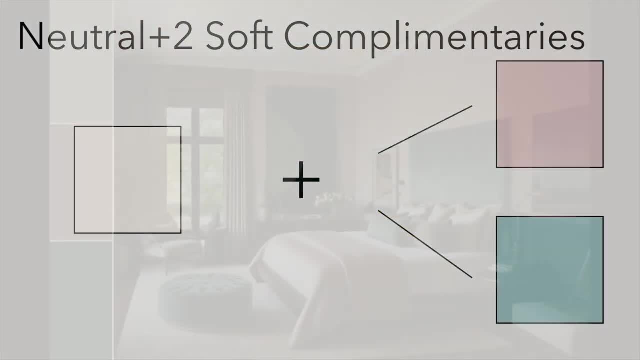 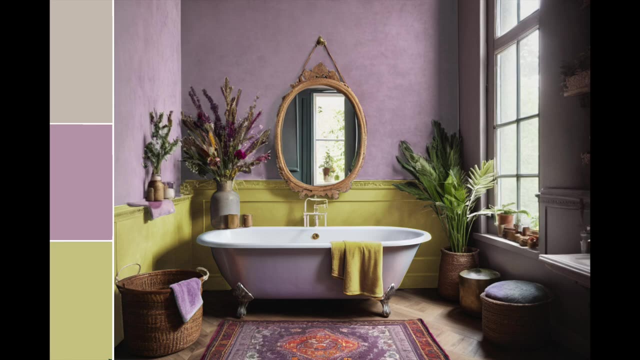 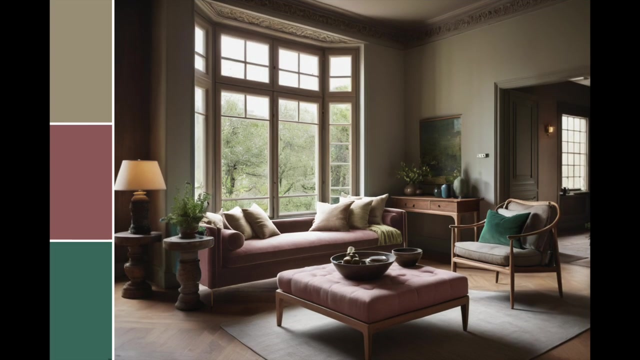 Integrating a neutral base with two soft complementary colors creates a more natural look. It creates an environment that balances the serene sophistication with subtle dynamism. This approach harmonizes the calming effect of neutrals with the intriguing contrast of complementary colors. However, by choosing softer tones, the contrast is more muted, resulting in a more harmonious. 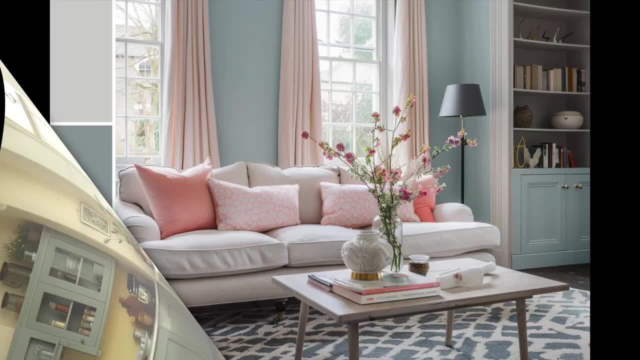 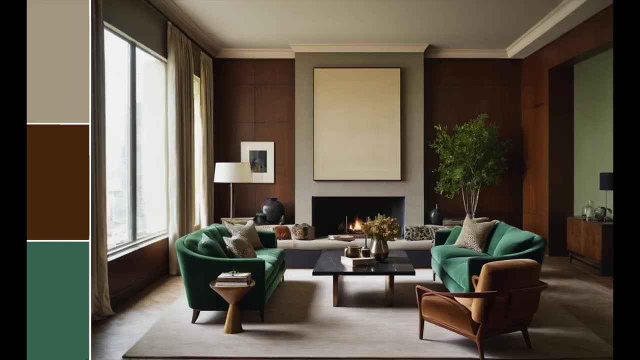 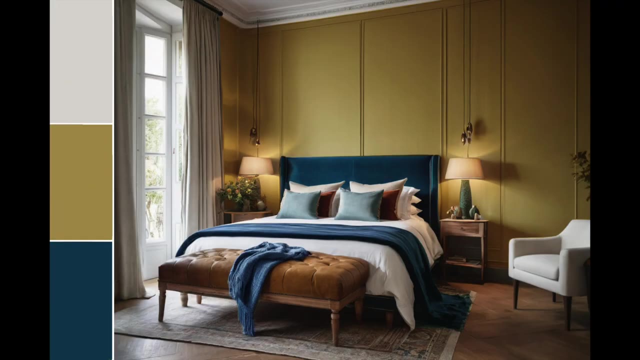 and less jarring effect. A neutral base with two bold complementary colors creates a striking and dynamic aesthetic. This palette combines the calming presence of the neutral base with the vibrancy of the neutralized colors. The combination of white, neutral and bold creates a clean, sophisticated and dynamic. 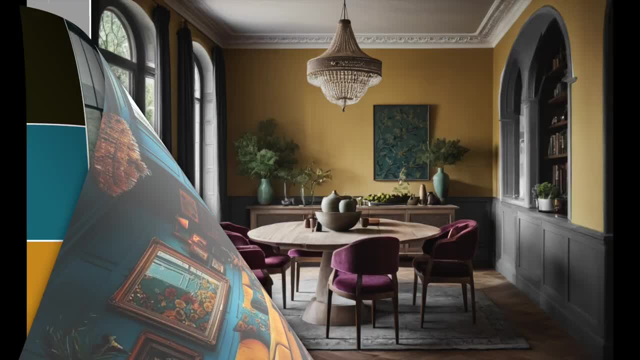 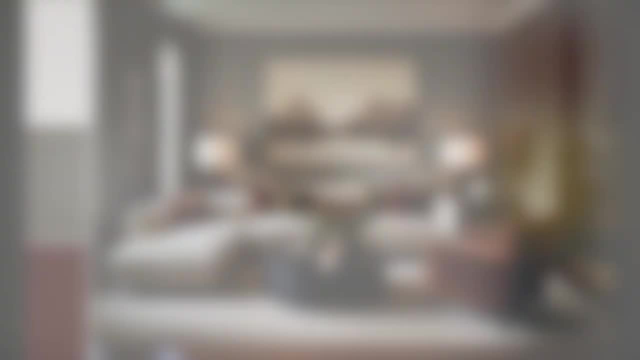 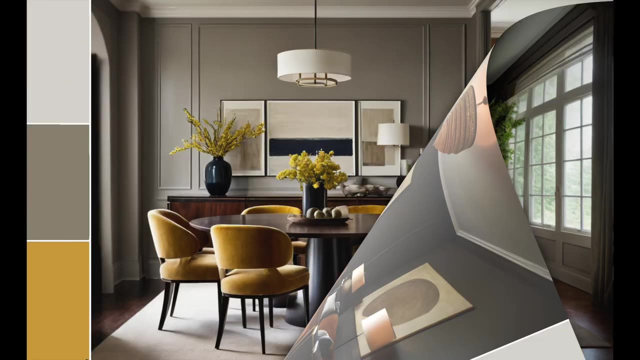 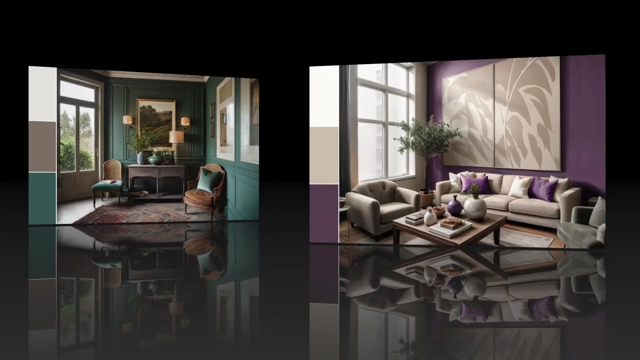 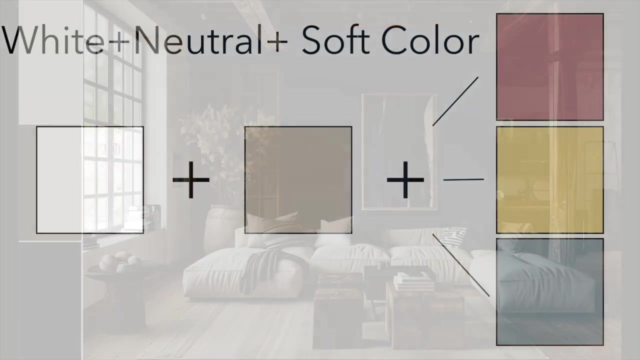 aesthetic. 8. Fine Coating. The combination of white, neutral and bold can create a clean, sophisticated and dynamic aesthetic. 9. Crispy White: 10. captivating. Incorporating a white, a neutral and a soft colour into your space creates a serene, gentle.